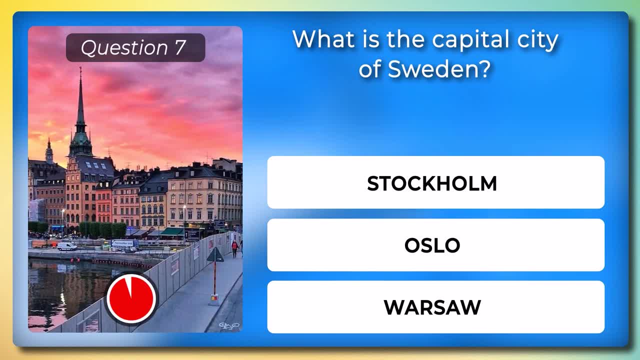 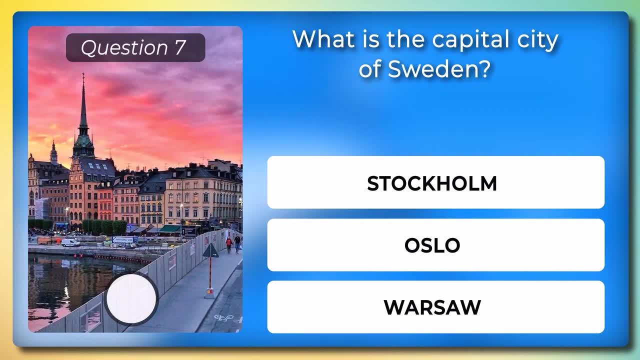 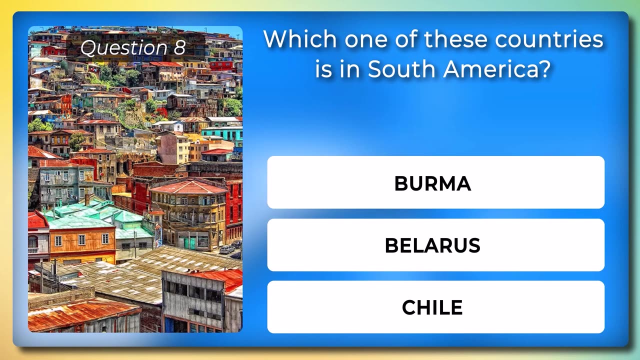 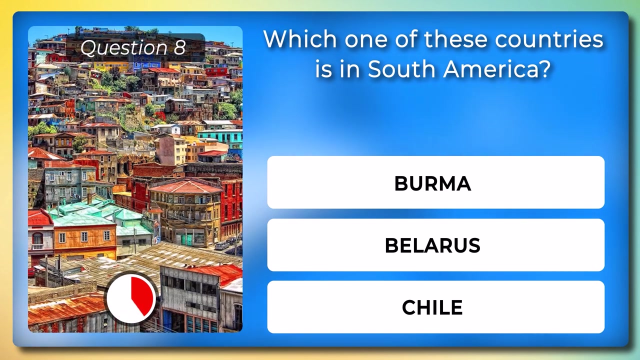 Sahara. What is the name of the biggest desert in Africa? Namib Gobi or Sahara? Namib Gobi or Sahara, Swahili Or Warsaw? The correct answer is Stockholm. Which one of these countries is in South America? Burma, Belarus or Chile? 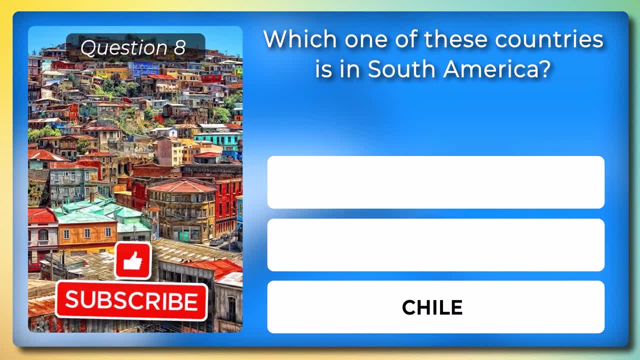 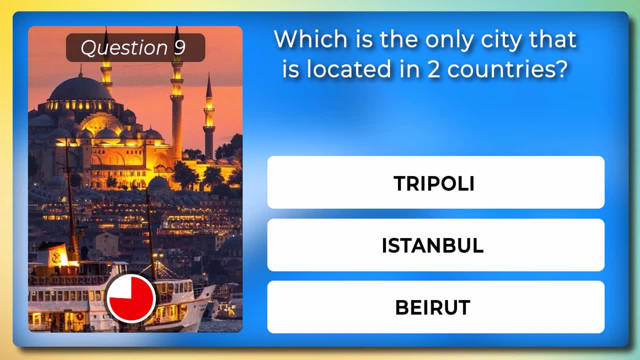 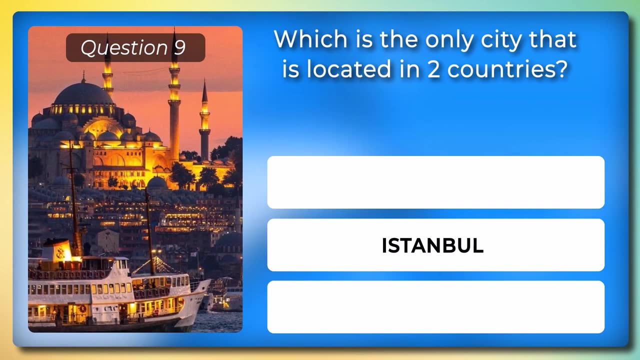 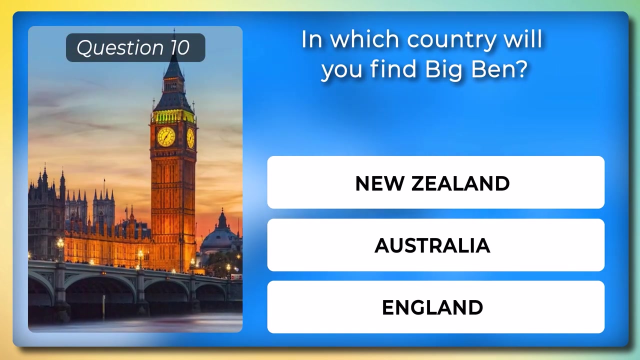 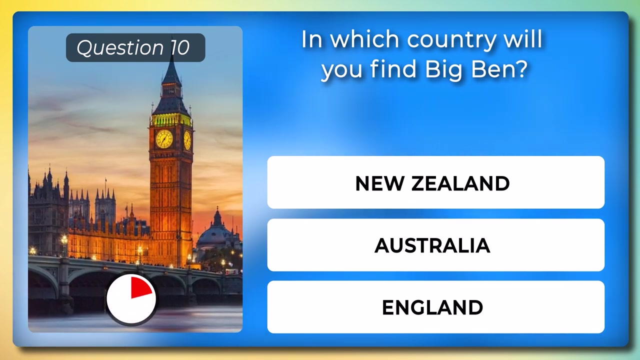 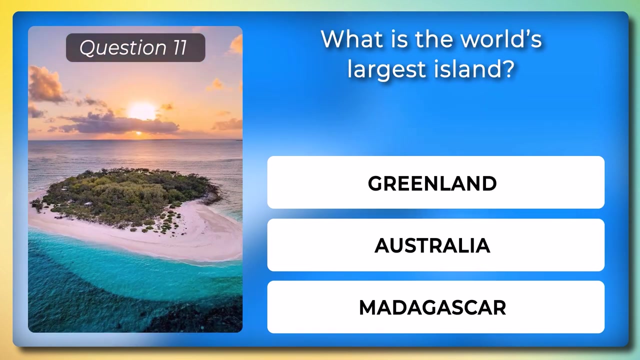 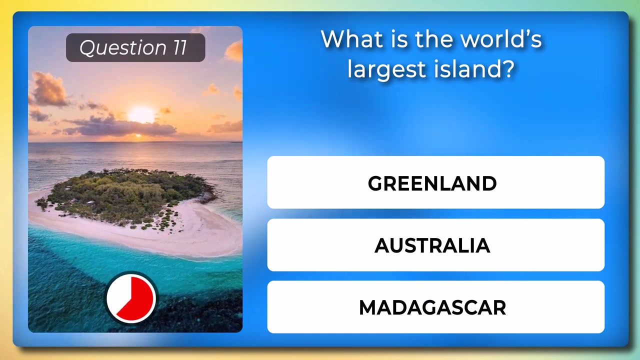 Chile, Which is the only city that is located in two countries: Tripoli, Istanbul or Beirut, Istanbul. In which country will you find Big Ben? New Zealand, Australia or England? In England, What's the world's largest island? Greenland, Australia or Madagascar? 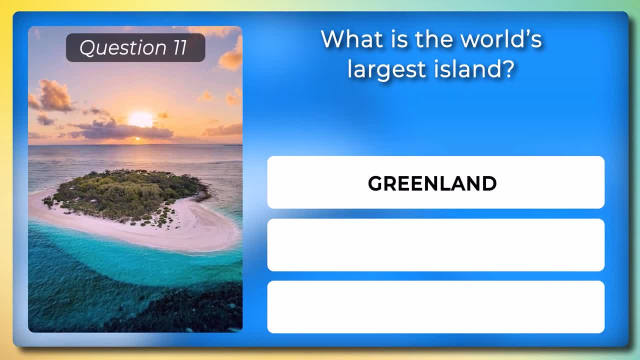 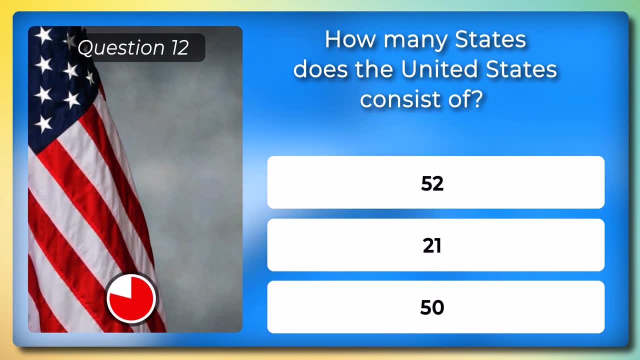 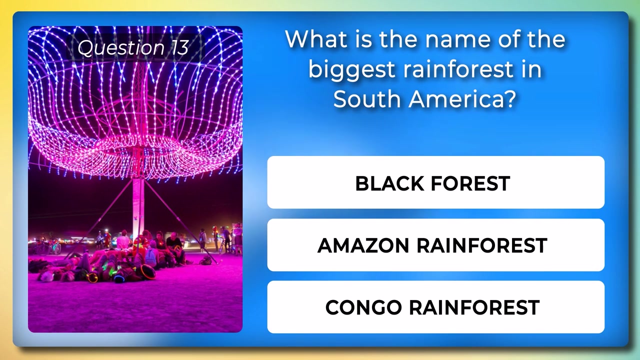 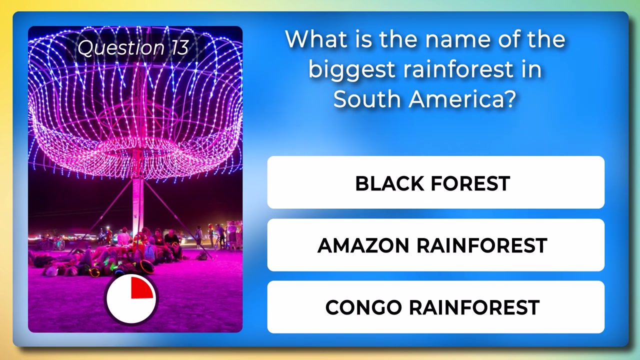 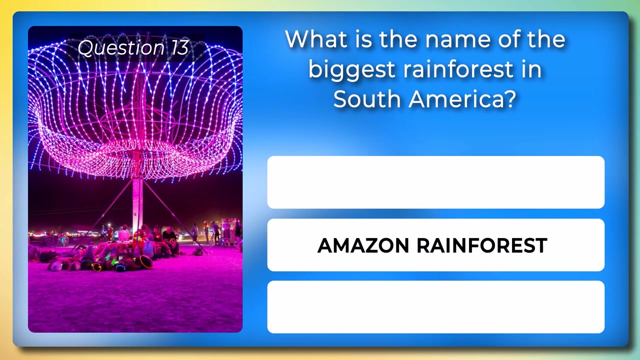 Greenland. How many states does the United States consist of? 52,, 21 or 50? 50? What's the name of the biggest rainforest in South America? the Black Forest, the Amazon Rainforest or the Congo Rainforest? The Amazon Rainforest? 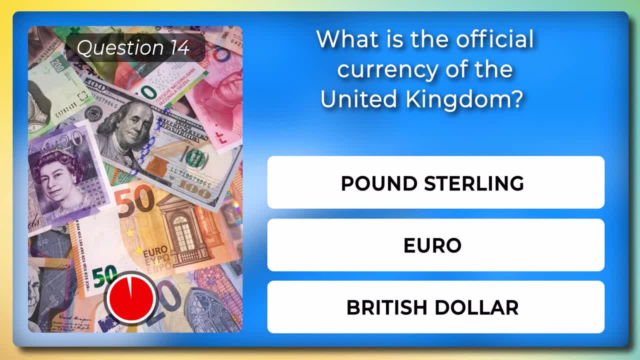 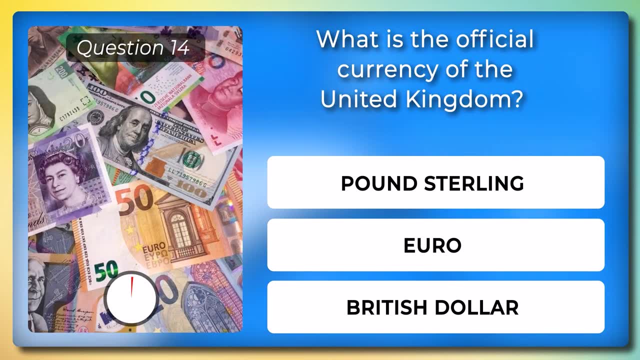 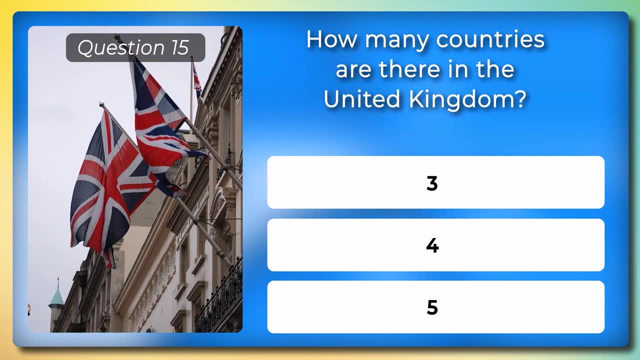 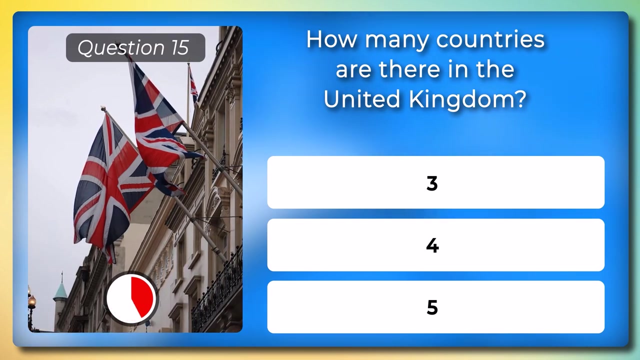 What's the official currency of the United Kingdom? Pound Sterling, the Euro or the British Dollar, The Pound Sterling. How many countries are there in the United Kingdom? Three, four or five? The correct answer is four. How many countries are there in the United Kingdom? 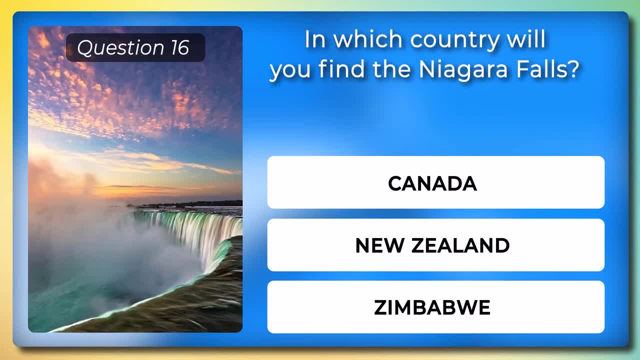 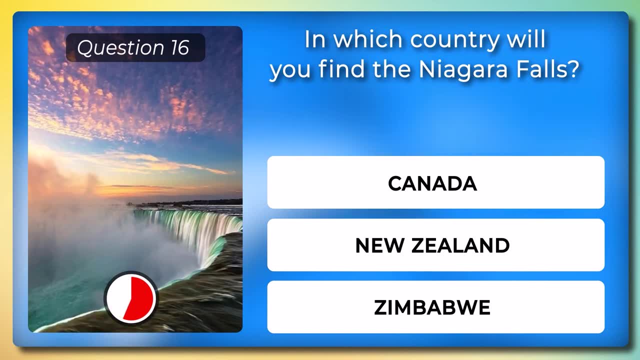 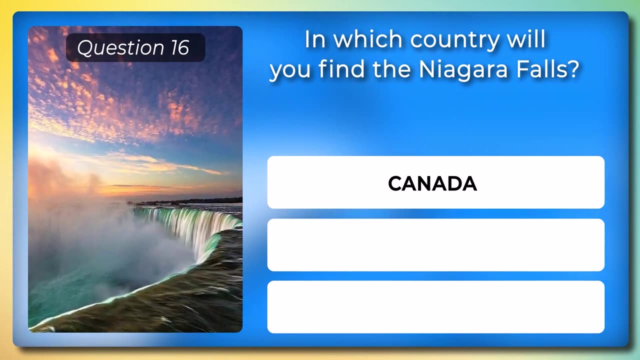 Three, four or five. The correct answer is four, Three, four or five. Where in the world was the United Kingdom founded as the capital city of Venezuela? What is it? whose capital city is it located in? Who created the Redeutschland? 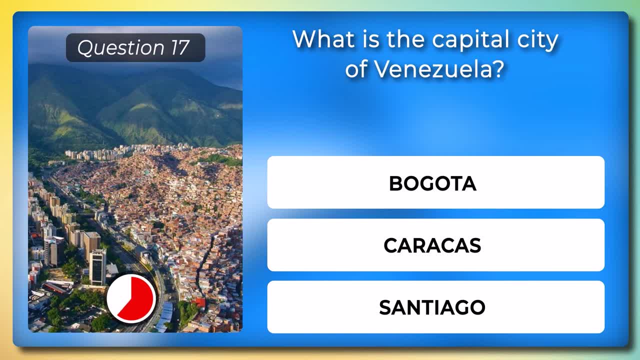 which is also called the 아직 abondoned city, Which are itsedral нем Simpson, Which희s is the industrial family member of Venezuela. In which country will you find the Niagara Falls? In which country will you find the Niagara Falls? Canada, New Zealand or Zimbabwe? 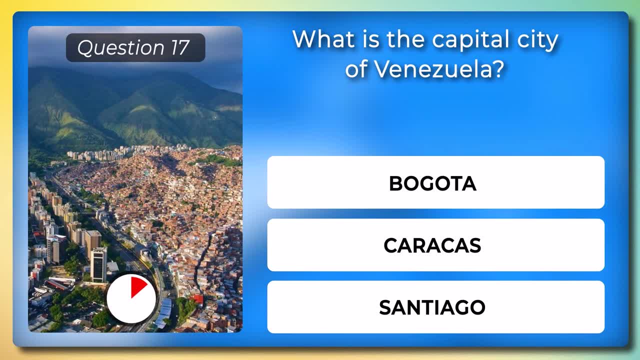 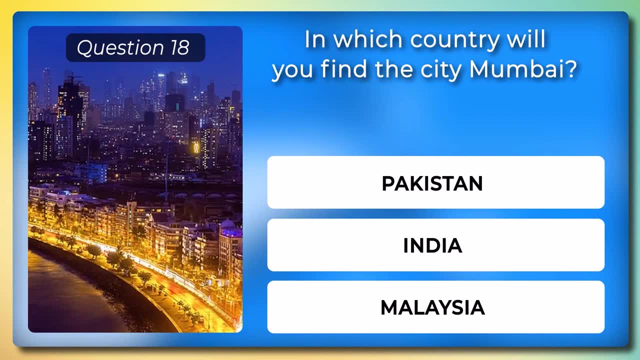 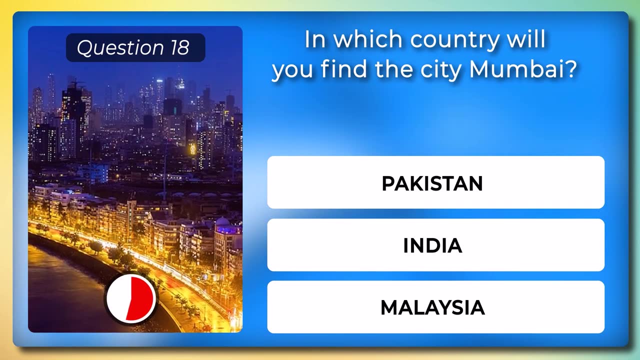 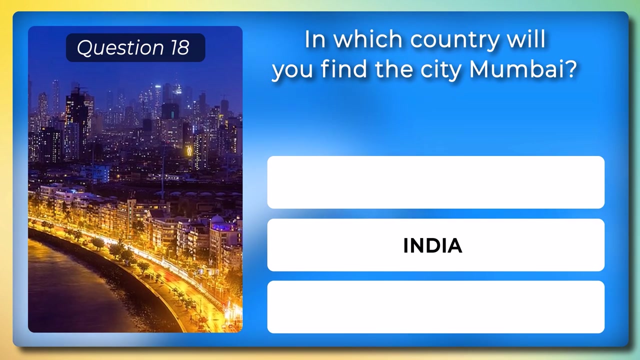 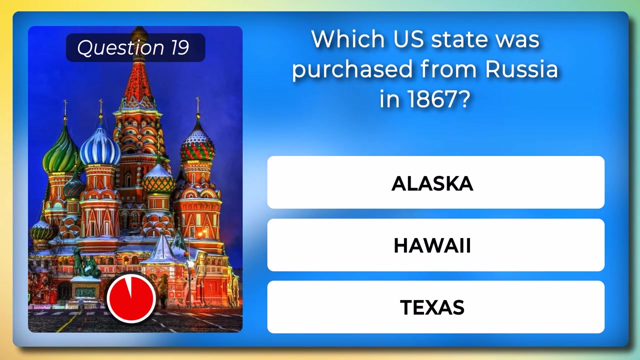 What's the capital city of Venezuela? Bogota, Caracas, Santiago, The capital city of Venezuela? In which country will you find the city? Mumbai, Pakistan, India or Malaysia? India? Which US state was purchased from Russia in 1867?? 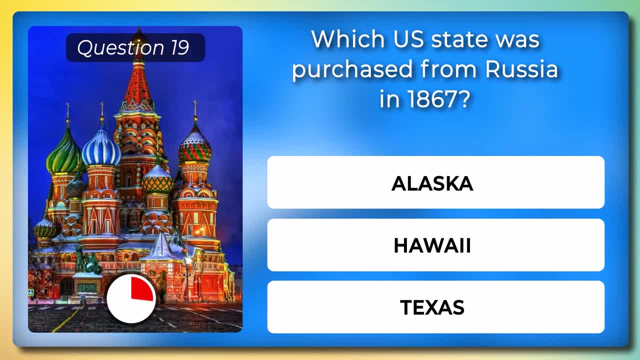 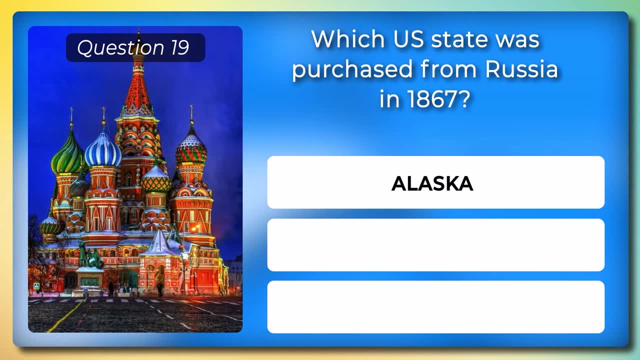 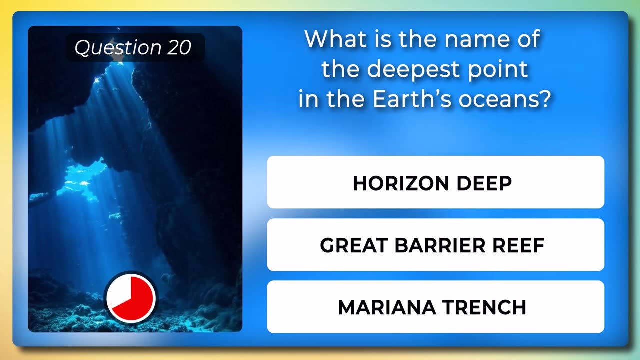 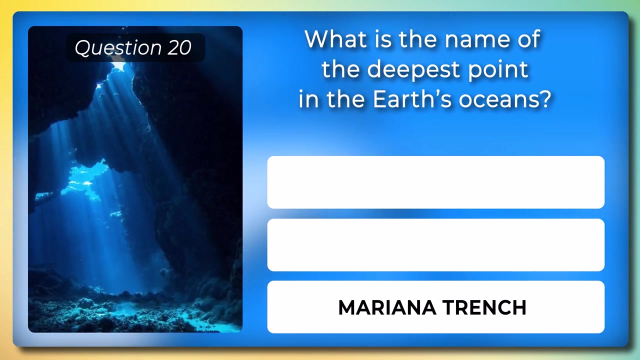 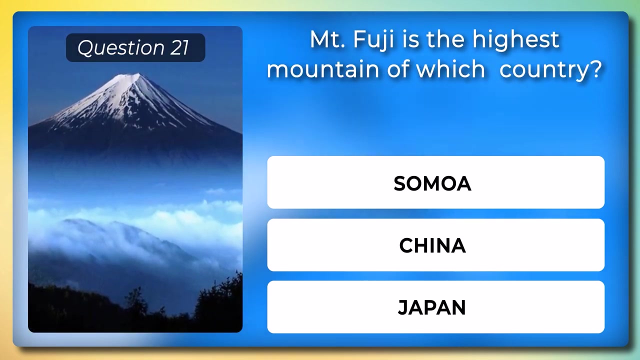 Hawaii or Texas, Alaska? What's the name of the deepest point in the Earth's oceans- Horizon Deep, the Great Barrier Reef or the Mariana Trench? The Mariana Trench, Mount Fuji is the highest mountain of which country? Samoa, China or Japan? 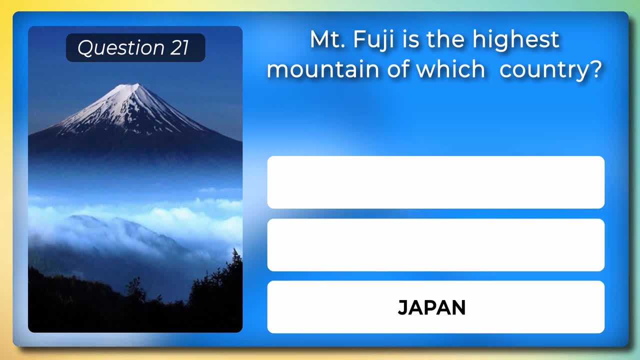 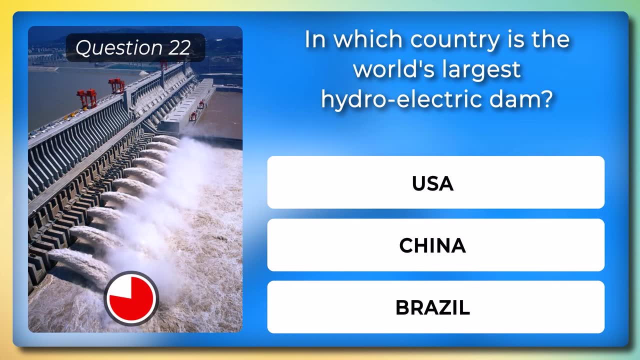 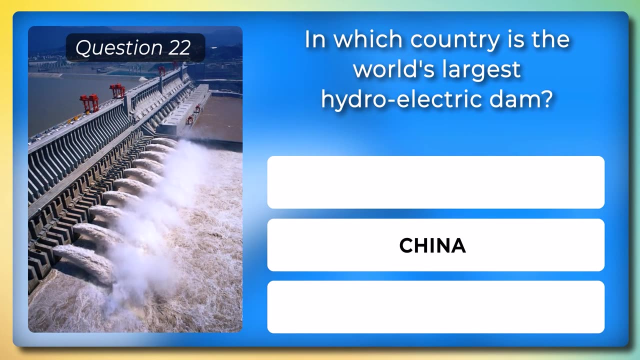 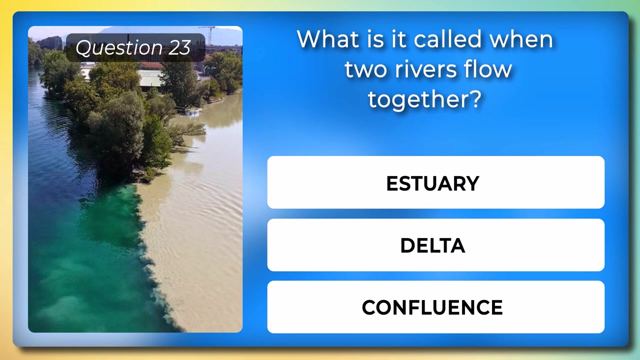 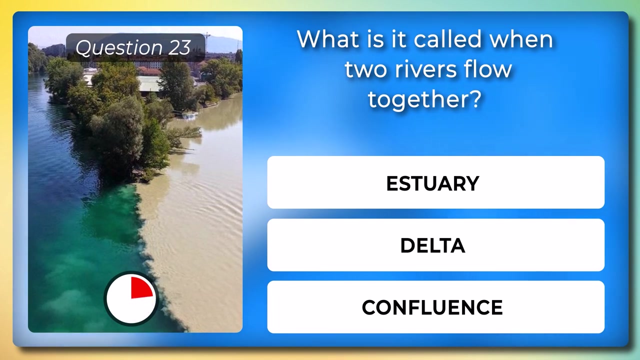 Japan. In which country is the world's largest hydroelectric dam? The USA, China or Brazil, China, China, China, China? What is it called when two rivers flow together: An estuary, a delta or confluence? A delta or a confluence.